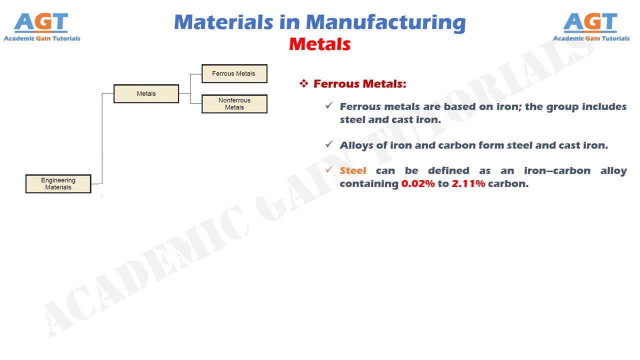 It is the most important category within the ferrous metal group. Its composition often includes other alloying elements as well, such as manganese, chromium, nickel and molybdenum, To enhance the properties of the metal. Applications of steel include construction bridges, I-beams and nails, transportation trucks, rails and rolling stock for railroads. 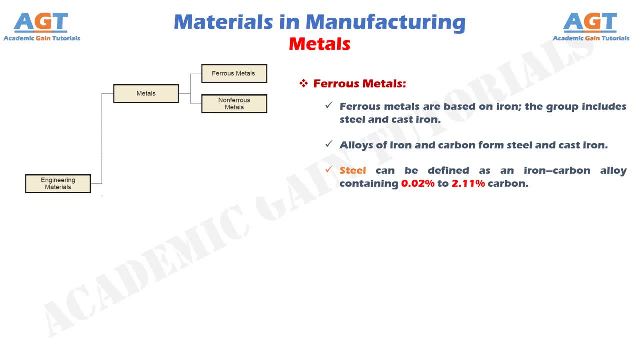 and consumer products, automobiles and appliances. Cast iron is an alloy of iron and carbon 2% to 4% used in casting, primarily sand casting. Silicon is also present in the alloy in amounts from 0.5% to 3%. 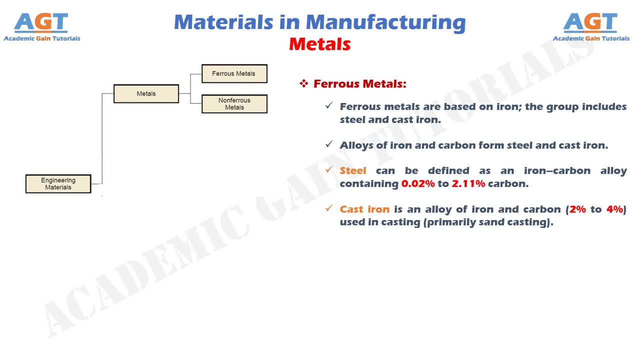 And other elements are often added also to obtain desirable properties in the cast part. Cast iron is available in several different forms, of which gray cast iron is the most common. Its applications include blocks and heads for internal combustion engines. Non-ferrous metals. 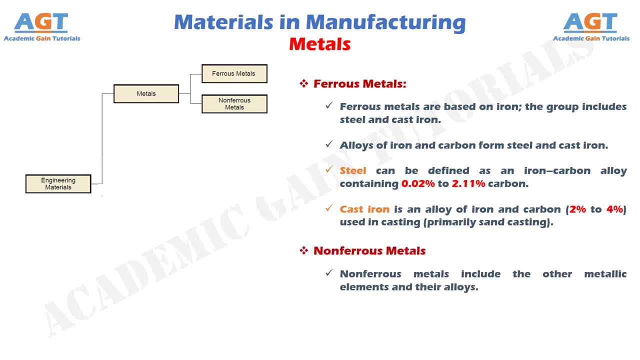 Non-ferrous metals include the other metallic elements and their alloys. In almost all cases, the alloys are more important commercially than the pure metals, The non-ferrous metals. The non-ferrous metals include the pure metals and alloys of aluminum, copper, gold, magnesium, nickel, silver, tin, titanium, zinc and other metals. 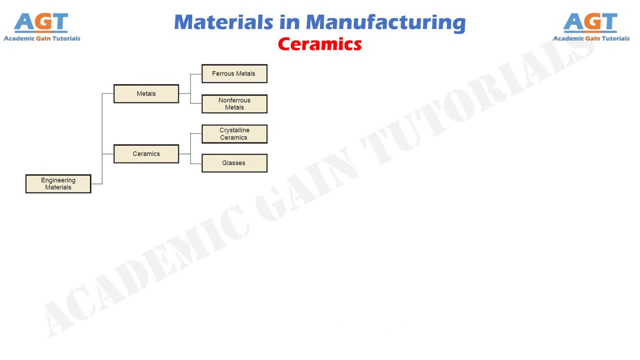 Ceramics. A ceramic is defined as a compound containing metallic or semi-metallic and non-metallic elements. Typical non-metallic elements are oxygen, nitrogen and carbon. Ceramics include a variety of traditional and modern materials. Traditional ceramics: 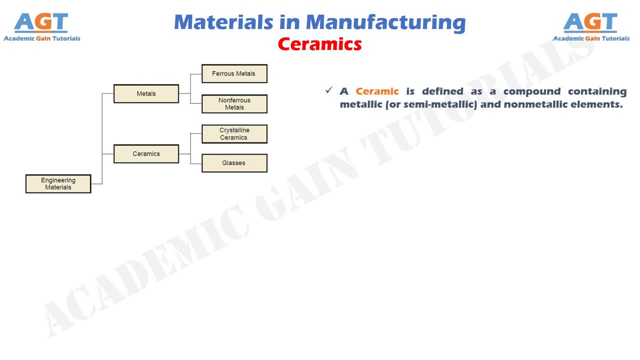 Traditional ceramics. Traditional ceramics, which have been used for thousands of years, include clay, which is abundantly available, consisting of fine particles of hydrous, aluminum, silicates and other minerals used in making brick tile and pottery silica, which is the basis for nearly all glass products. and 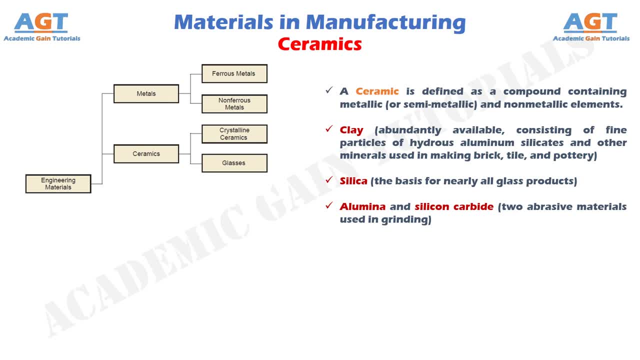 alumina and silicon carbide, which are two abrasive materials used in grinding. Modern ceramics include some of the preceding materials, such as alumina, whose properties are in-house are enhanced in various ways through modern processing methods. Newer ceramics include carbides- the metal carbides, such as tungsten carbide and titanium carbide, which are widely used as cutting tool materials. 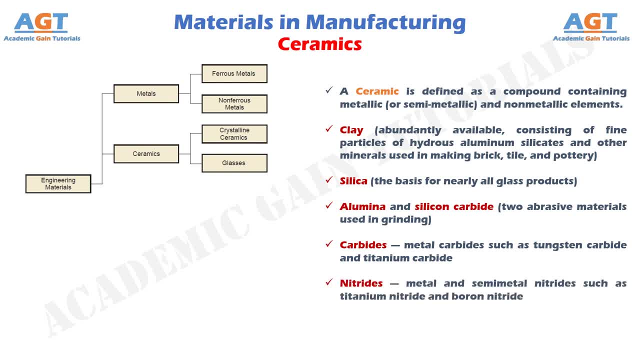 and nitrides: the metal and semi-metal nitrides, such as titanium nitride and boron nitride, used as cutting tools and grinding abrasives For processing purposes. ceramics can be divided into crystalline ceramics and glasses. Different methods of manufacturing are required for the two types. 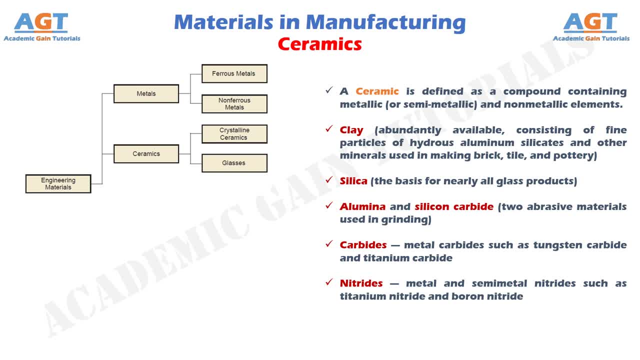 Crystalline ceramics are formed in various ways from powders and then fired heated to a temperature below the melting point to achieve bonding between the powders. The glass ceramics, namely glass, can be melted and cast and then formed in processes such as traditional glassblowing. 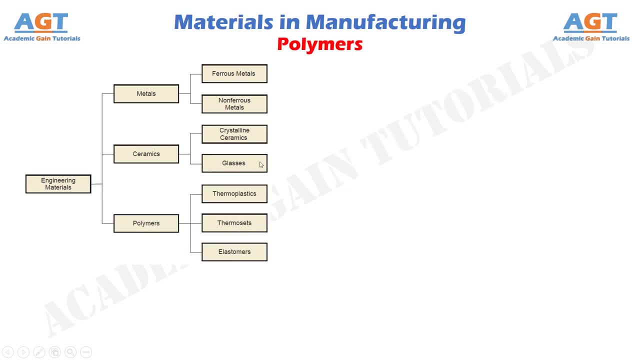 Polymers. A polymer is a compound formed of repeating structural units called mers, whose atoms share electrons to form very large molecules. Polymers usually consist of carbon plus one or more other elements, such as hydrogen, nitrogen, oxygen and chlorine. 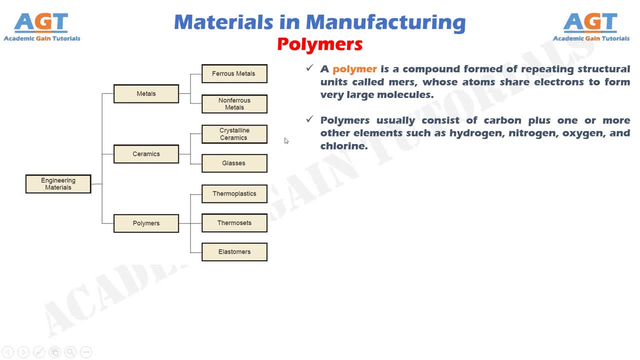 Polymers are divided into three categories: Thermoplastic polymers, Thermosetting polymers and Elastomers. Thermoplastic polymers can be subjected to multiple heating and cooling cycles without substantially altering the molecular structure of the polymer. Common thermoplastics include polyethylene, polystyrene, polyvinyl chloride and nylon. 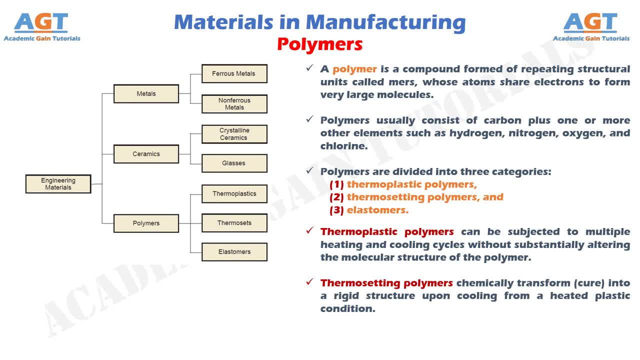 Thermosetting polymers chemically transform into a rigid structure upon cooling from a heated plastic condition, hence the name thermosetting. Members of this type include phenolics, amino resins and epoxies. Although the name thermosetting is used, some of these polymers cure by mechanisms other than heating. 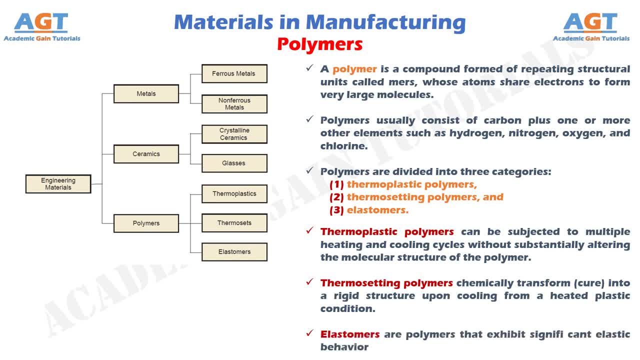 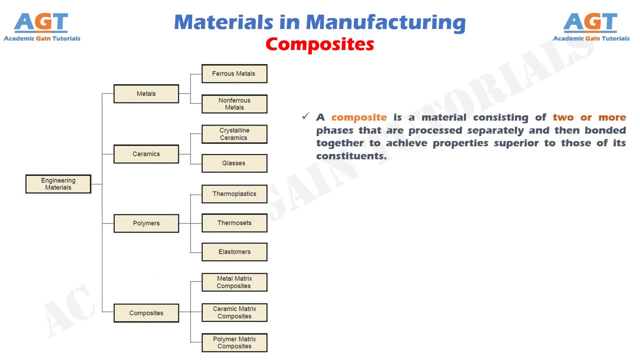 Elastomers are polymers that exhibit significant elastic behavior, hence the name elastomer. They include natural rubber, neoprene, silicone and polyurethane Composites. Composites do not really constitute a separate category of materials. they are mixtures of the other three types. 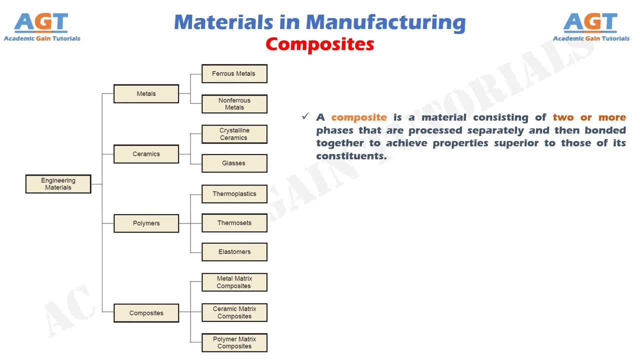 A composite is a material consisting of two or more phases that are processed separately and then bonded together to achieve properties superior to those of its constituents. The term phase refers to a homogeneous mass of material, such as an aggregation of grains of identical unit cell structure in a solid metal.